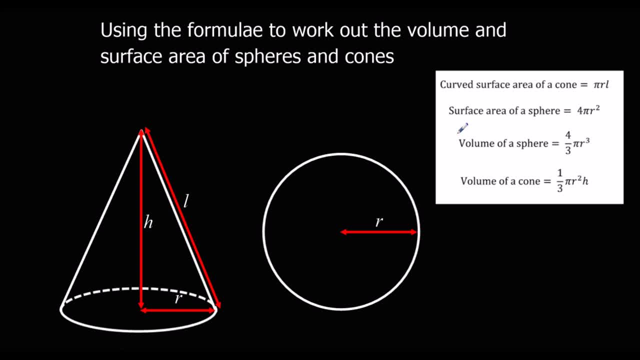 pi r cubed. So we just apply these formulas and that tells us how to work out the volume and surface area. So here I've got a sphere. So if I want to work out the volume, I just take the formula. So it's 4 over 3 times pi r cubed. In this case, r is 5. So it's 4 over. 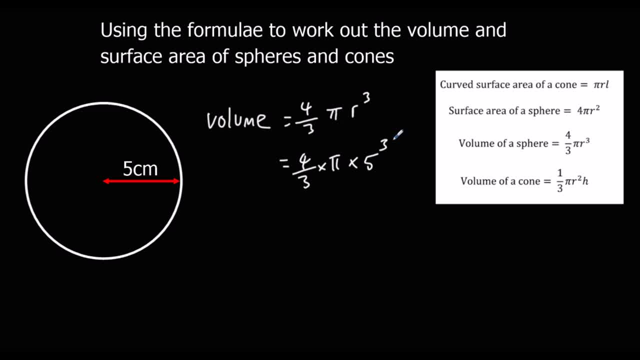 3 times pi times 5 cubed And you can just type that in the calculator and that gives us 500 over 3 pi, 4 is a decimal, we can have 523.6 its volume, so centimetres cubed to 1 dp The surface. 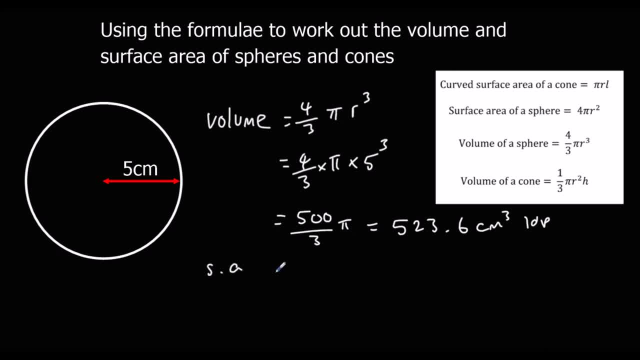 area. we just use the other formula. So surface area of a sphere is 4 times pi times r squared. In this case r is 5.. So 4 times pi times 5 squared, That gives us 100 pi. So as a decimal that's 314.2cm2 squared to 1 dp. 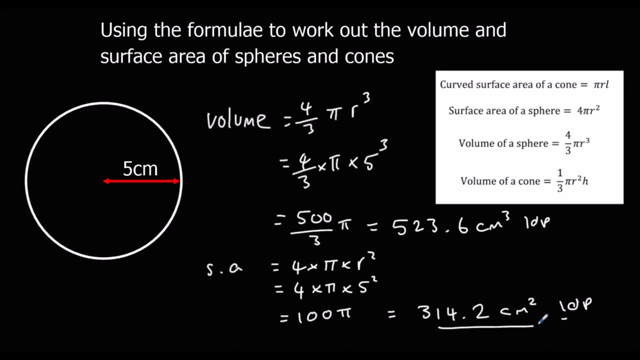 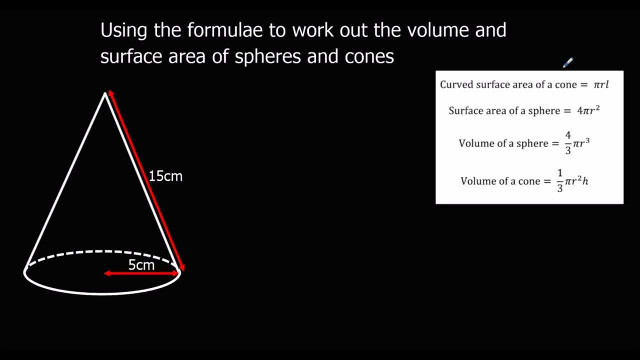 OK, so we've got a cone here, the curved surface area of a cone. so if I want to work out, actually, let's do volume first. So the volume, that's the easier one. in this case its 1 thirds times pi r-squared. 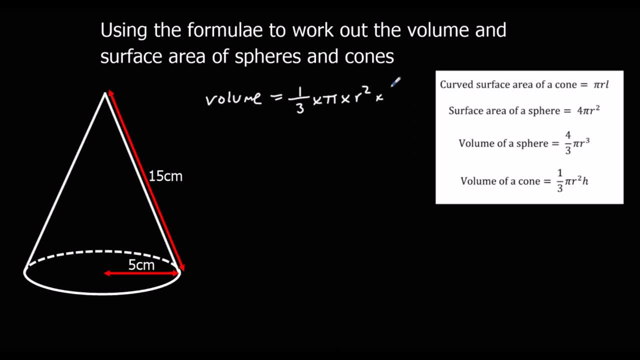 4 times pi r-squared times r squared, So 1 third times pi r squared. So that's just 1 third of the surface area, 1 third of the r squared times h, which is one third pi times five squared. but we don't actually know the. 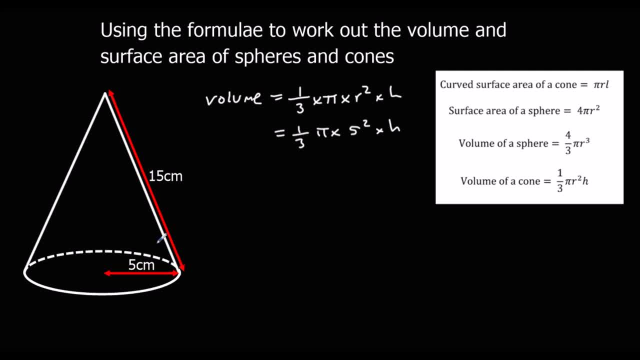 h in this case. so I'll just leave times h there for now. we know l, we know the curved one, but we don't know this vertical height. so what we've actually got here is a right angle triangle and it's a Pythagoras problem. so 15, 5 and our unknown here. so because of 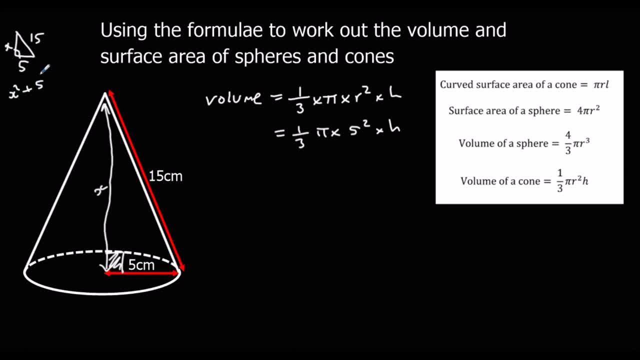 Pythagoras. we know that our unknown plus 5 squared equals 15 squared. so our unknown squared plus 25 equals 225. uh, so x squared equals 200 and our unknown is root 200. yeah, we'll just leave that as root 200. so it's one third pi times five squared times root 200. so then we can type that in. 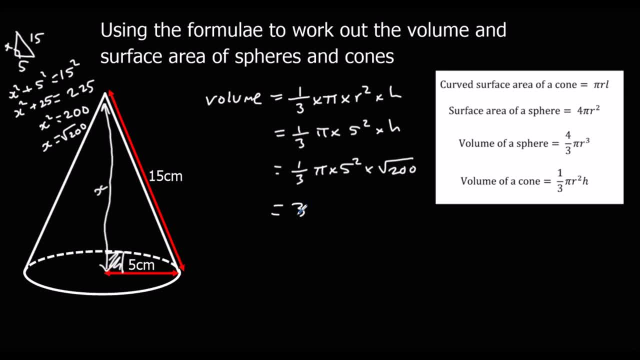 the calculator and that gives us an answer of 370.2 centimeters cubed and that's the one decimal place razor. the surface area with the curved surface area and the total surface area is the area of the circle. so obviously we do with the circle plus the curved surface area, so the 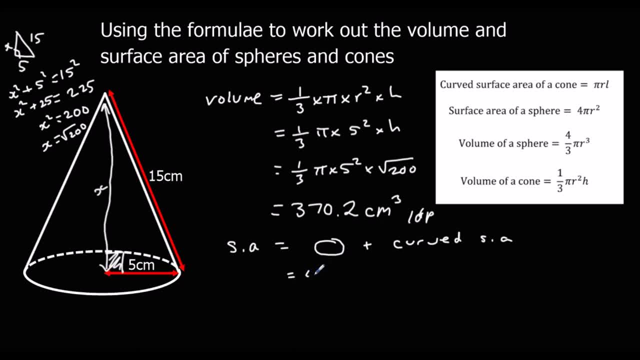 array of the circle is pi times R squared, pi times 5 squared, in this case, plus the curved surface area, which is pi times R times L, so pi times 5 times 15. so that's going to be 25 pi 6.9 in the nth cercertiously 0.66 in the eark of the surface area, plus r times. 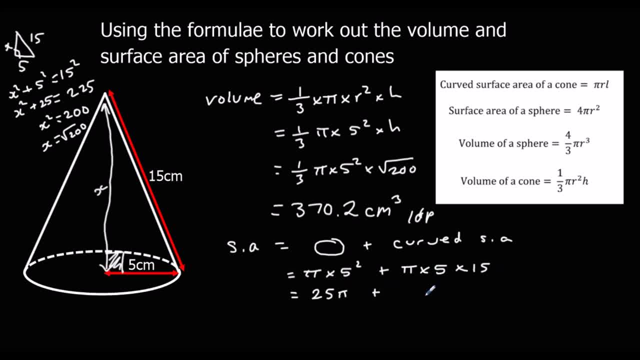 lice, whose area of the circa circle plus the khoenigsegg's area squared, so we said r times plus 515 to 75,, 75 pi, so that's 100 pi, So that's 314.2 centimetres squared and that's the 1dp. 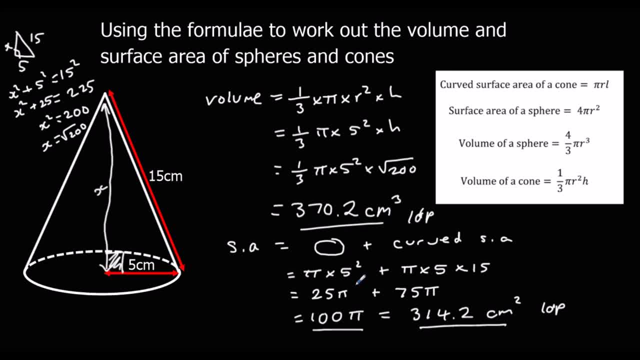 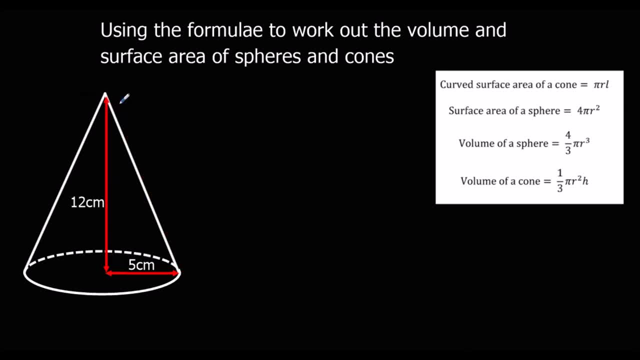 So either of those two answers 100 pi or 314.2.. Okay, this time they've given us the vertical height, they haven't given us the L, So we're going to have to work that one out to do the curved surface area. 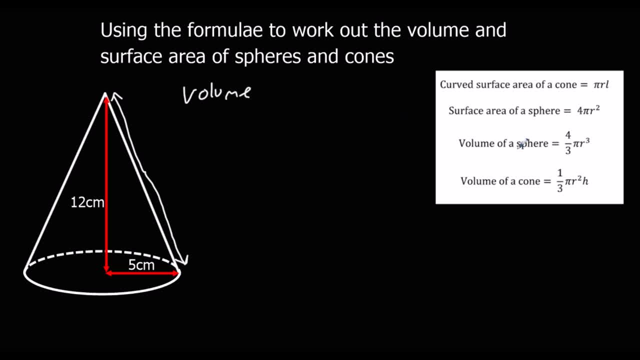 But we'll start with the volume. That's 1 third times pi r squared h, In this case 1 third times pi times 5 squared Times 12.. And that is 100 pi. Okay, so 314.2 centimetres cubed to 1dp. 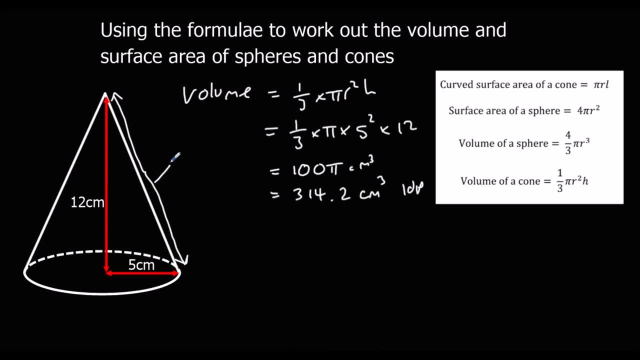 The L to find the curved surface area. we need to find L, and that's another Pythagoras problem. So we've got 5.. 12,, 12, and L here. 12 squared plus 5 squared equals L squared. 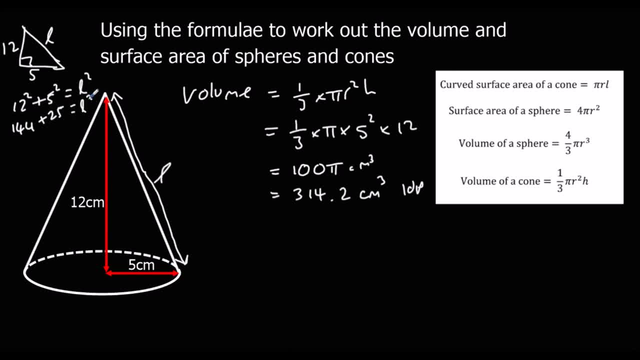 144 plus 25.. 169 equals L squared, So L is 13 centimetres. 13 centimetres, So we've got curved surface area as pi r L, Which is pi times 5 times 13,, which is 65 pi. 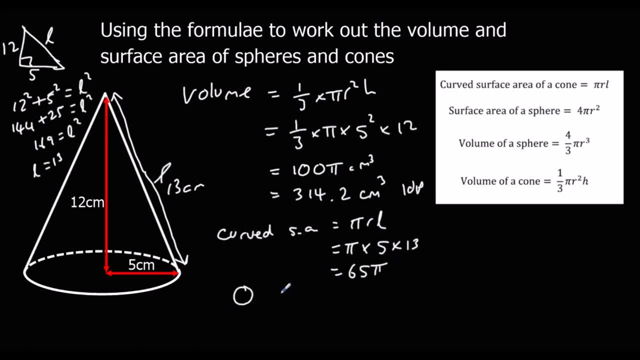 And we've got the circle which is pi times r squared, So 25 pi. So that means that adds up to 90 pi. So the total surface area is 90 pi, Or 282.7 centimetres squared To 1dp. 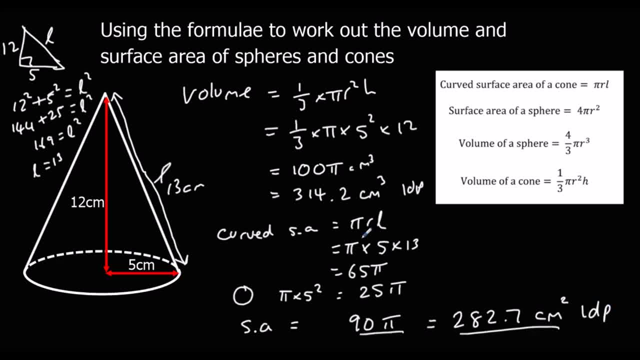 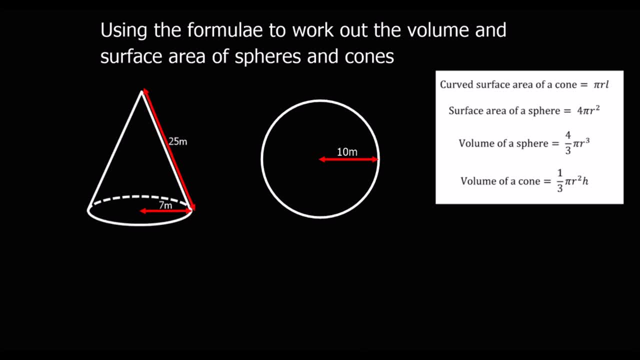 Okay, here's two questions for you to try So see if you can work out the volume and surface area for this cone and this sphere. Okay, so if we look at the cone here, we can see that we need to work out the h to work out the volume. 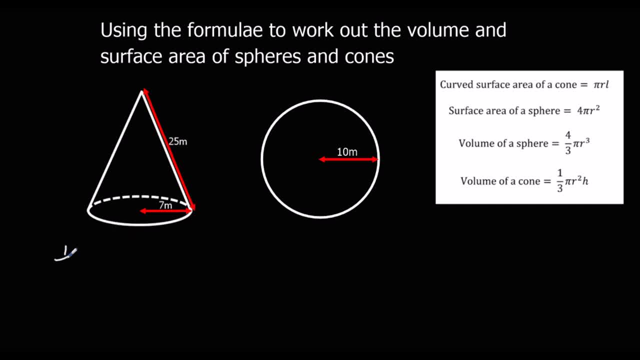 Because volume is 1 third pi r squared h. So we use Pythagoras to find this length. So it's going to be 7 squared plus h squared equals 25 squared And that gives us h squared equals 25 squared minus 7 squared, which is 576.. 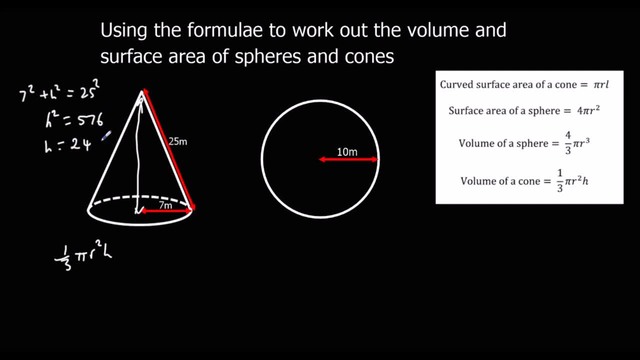 And h is 5.. So that gives us root 576, which is actually 24.. So 24 metres is the height. So the volume is 1 third times pi, times 7 squared times 24.. And we type that in the calculator and we get 392 pi, or as a decimal, that's 1231.5 to 1dp.